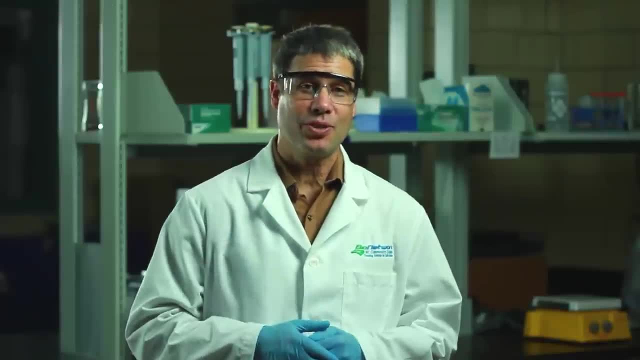 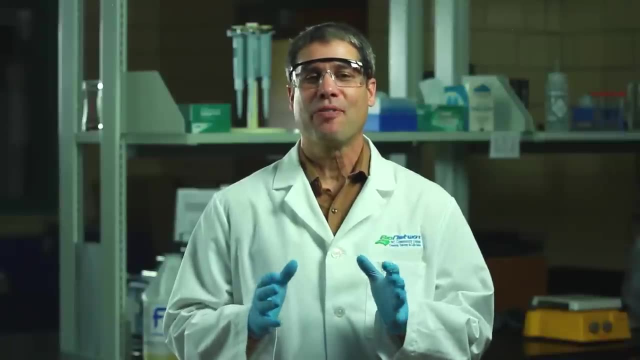 in the lab can help prevent serious, even fatal, injuries. Often you'll be working with chemicals that could harm you if they come into contact with your skin, So the best way to prevent skin exposure is to wear clothes that cover your entire body- Shorts and sandals. 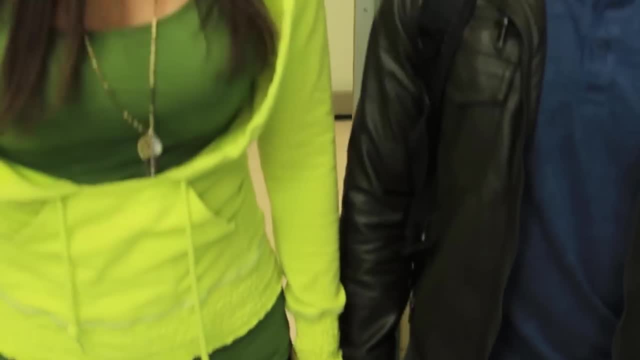 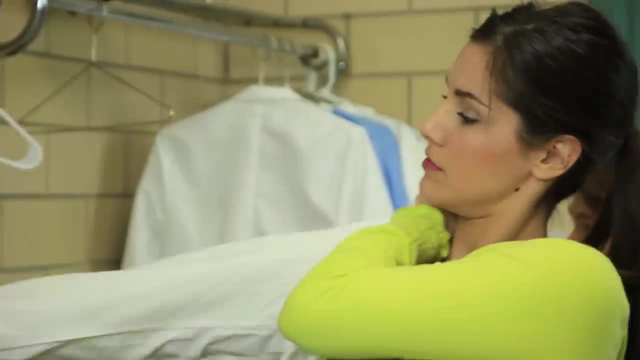 leave your skin exposed, so instead wear long pants and closed-toed shoes. Remove jewelry before entering the lab and tie back long hair. Bring only the things that you need into the lab. Leave all personal items like backpacks, purses or jackets outside, so they 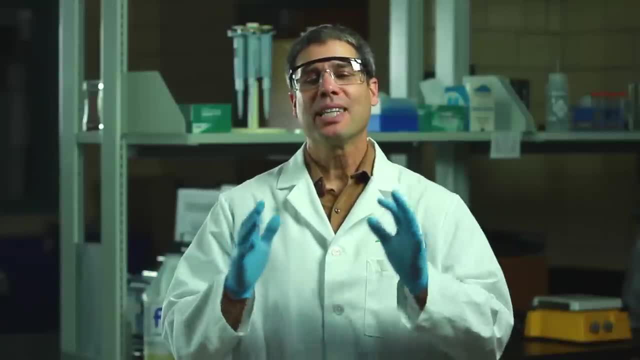 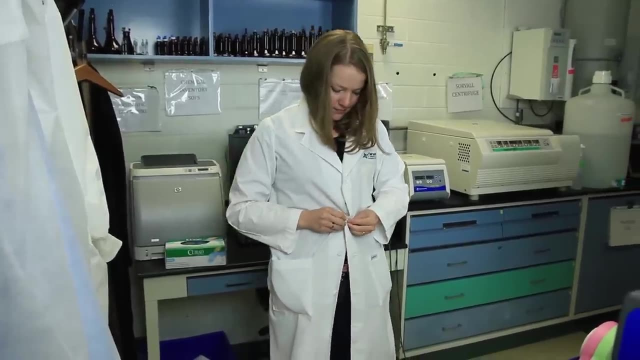 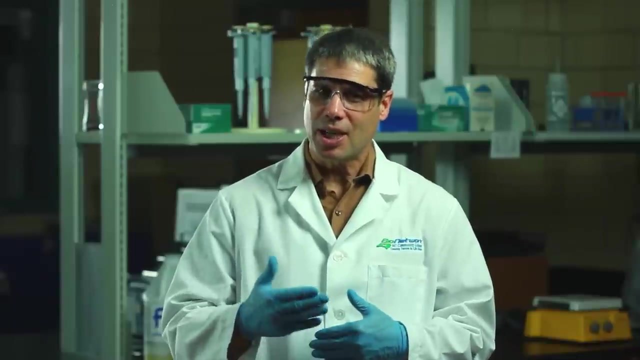 don't become contaminated. Now that you're properly dressed for the lab, let's take a look at Personal Protective Equipment, or PPE. For general lab work, a lab coat, safety glasses or goggles, and gloves are required. Always button your coat and try to keep the cuffs. 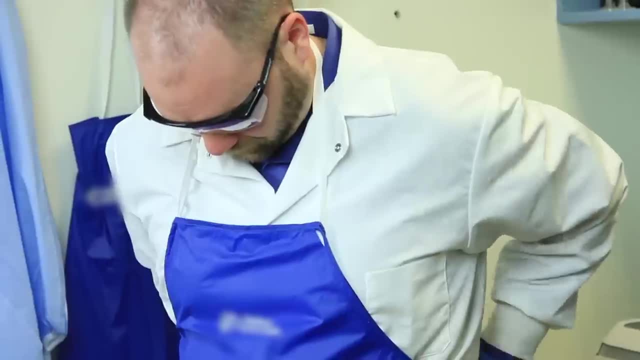 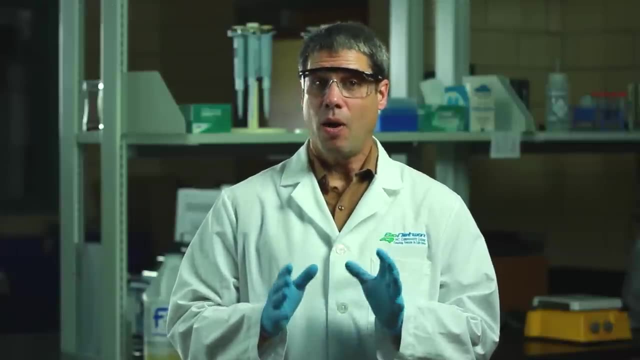 tucked into your gloves. Wear a chemical apron if you're working with splash hazards, volatile or reactive solutions. Safety glasses can protect your eyes from flying debris. However, these glasses won't protect you from splash hazards. That's why you may need to. 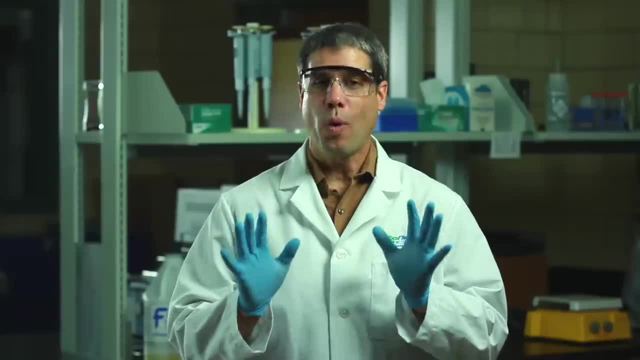 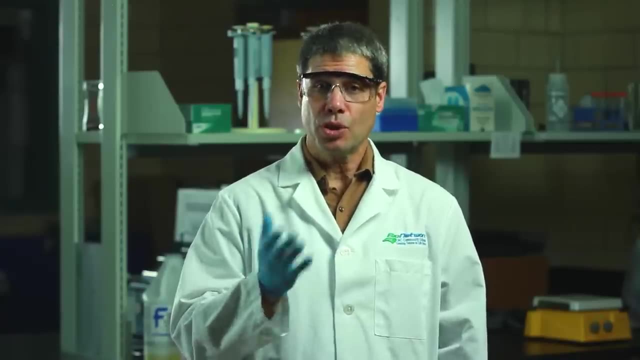 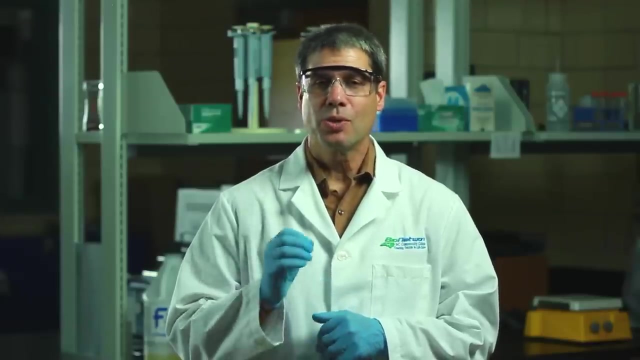 wear chemical-resistant safety goggles. Always wear gloves in the lab. Be sure to choose the most appropriate type. You need gloves that are resistant to the chemicals you'll be handling. These gloves are non-absorbent. Even so, chemicals can leach through over time, so it's a good idea to change your gloves. 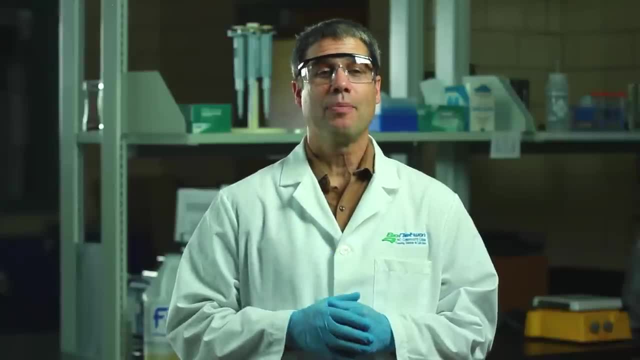 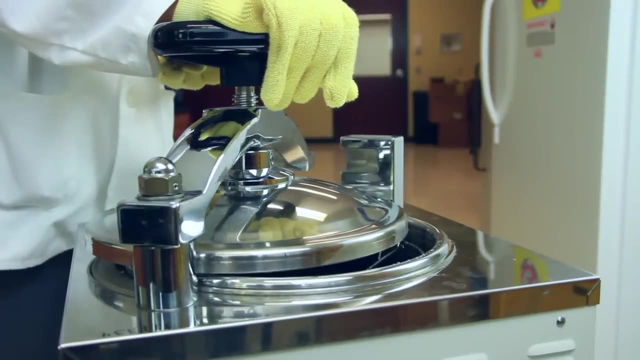 and wash your hands frequently, especially if they've come into contact with chemicals. Thermal and puncture-resistant gloves are used for handling extremely hot or cold materials, such as when using the autoclave, handling dry ice or handling sharps Some chemicals. 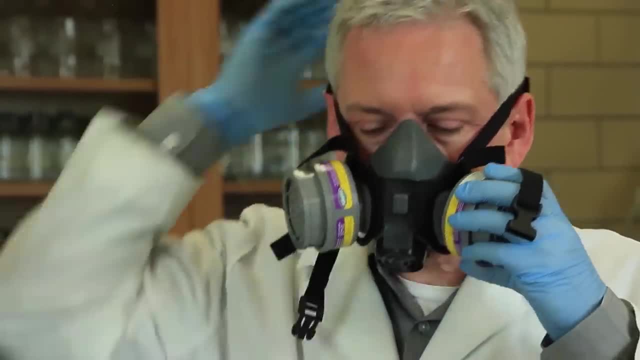 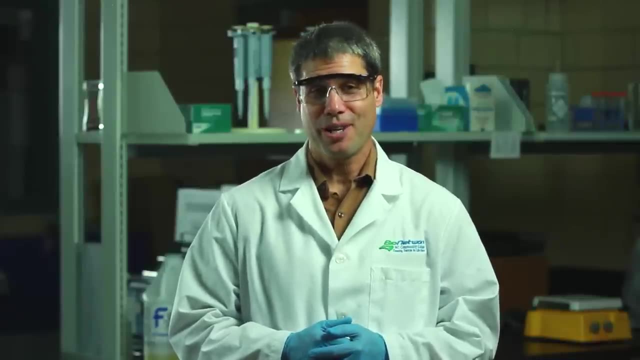 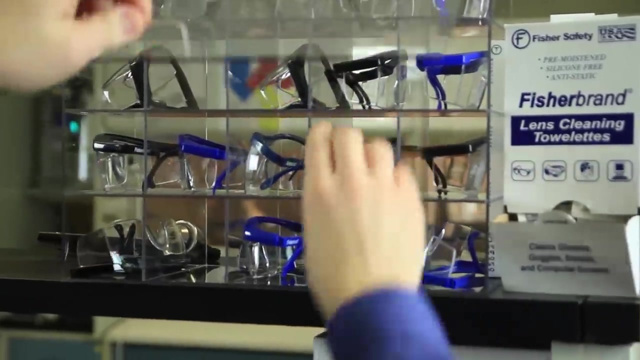 produce dangerous vapors. A respirator can protect you. However, by law you must first complete the proper training, So ask your lab manager or instructor about respirator training. Always remove PPE and wash your hands before leaving the lab and entering public areas, And be aware that you.